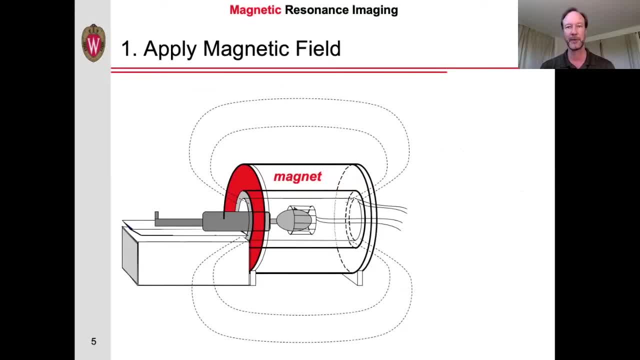 resonance and imaging. First, we place the person to be scanned into a large magnet. This magnet consists of coils of wire, as shown here in this schematic of an electromagnet. The magnets used for medical imaging typically have a strength of about 1.5 to 3 Tesla. This 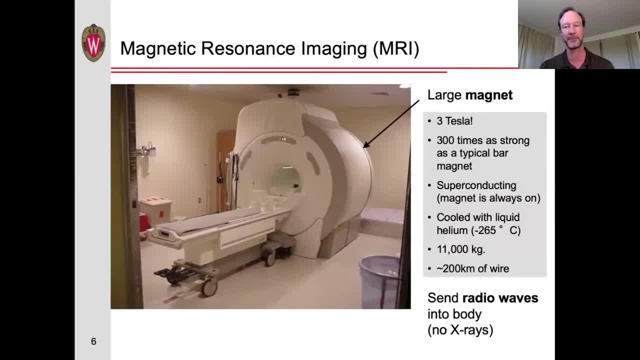 is about 300 times as strong as a typical bar magnet. It consists of about 200 kilometers of wire and weighs up to 11 tons. The wires used in MRIs is superconducting, meaning it has no resistance as long as they are just kept. 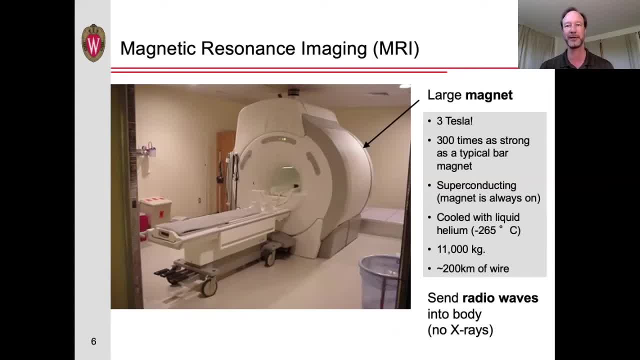 very cold. MRIs are therefore cooled with liquid helium at about minus 270 degrees Celsius. In addition, because the wires are superconducting, the current flows through these wires even without applying any external power. As a result, the MRI magnet is always on. 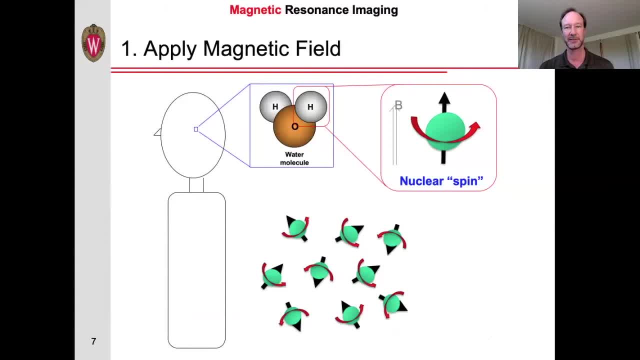 Next slide. Third, Certain atoms, such as hydrogen, have a property called nuclear spin. In the absence of a magnetic field, these spins point in random directions, as illustrated here. However, in the presence of a magnetic field, these spins either align or anti-align themselves. 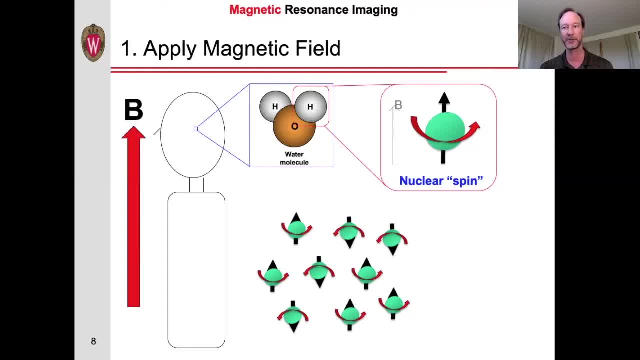 with the magnetic field. One atom in particular whose hydrogen likes to align itself with the magnetic field is hydrogen, and especially hydrogen bound in the form of water. These, These spins, process or spin around the magnetic field with a specific frequency: omega that. 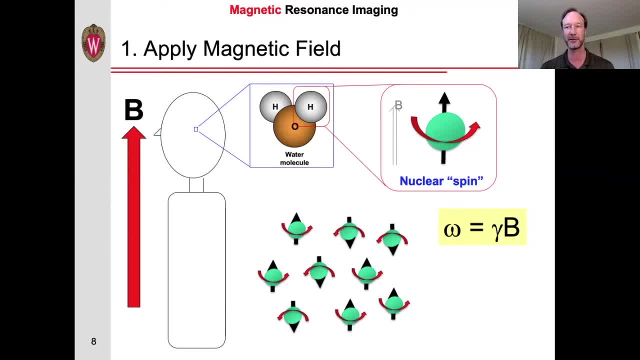 is directly proportional to the strength of the magnetic field B that they experience. Slightly more spins align themselves with the magnetic field instead of anti-align themselves. This results in a net magnetization. Now this magnetization is extremely small. Fortunately, water is one of the most abundant molecules in the human body. however, the 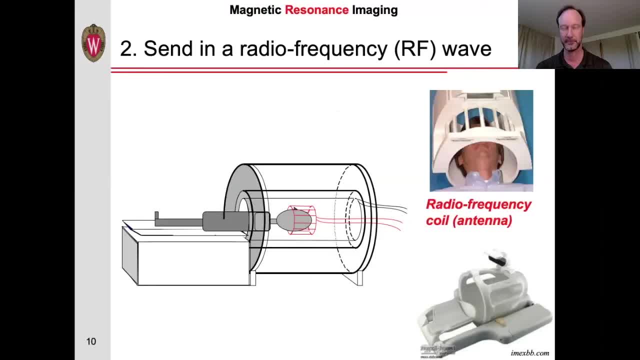 magnetization is still too small to detect directly. The way we detect this small magnetization is by using radio waves and resonance. A radio wave is sent into the part of the body we want to image using a radio frequency or RF coil. 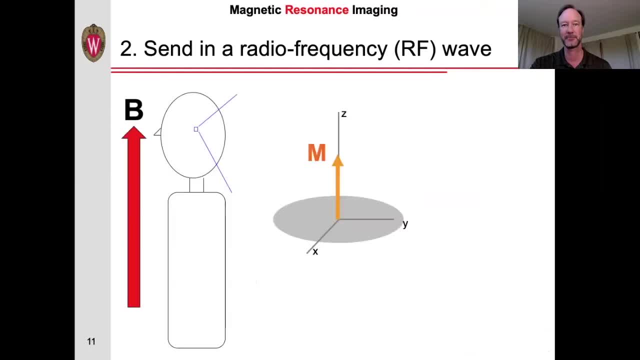 These coils can have a variety of shapes and sizes. When a radio wave of a specific frequency is sent into the body, the magnetization of the radio wave is very small. The magnetization is tipped away from being aligned with the main magnetic field. 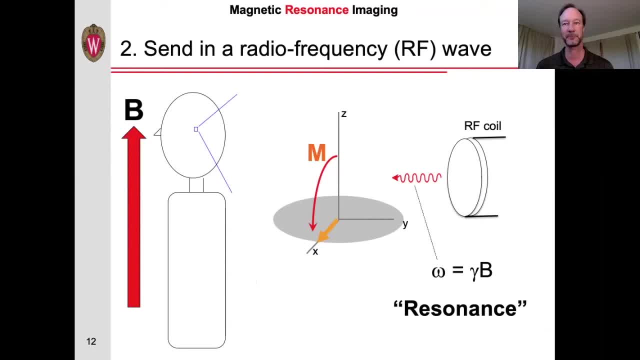 The frequency of the radio wave necessary to tip the magnetization is the same as the precession frequency of the spins. This is why we call it magnetic resonance imaging. The radio wave is then turned off and the magnetization precesses or rotates around. 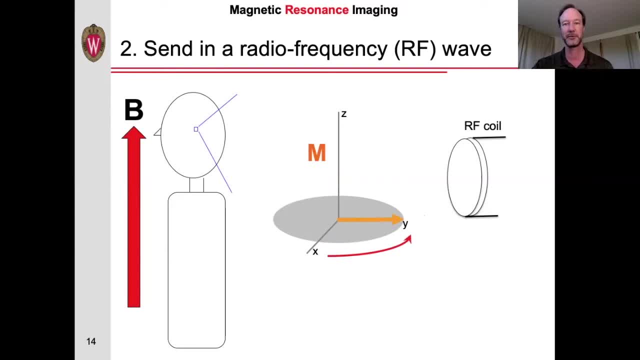 the direction of the main magnetic field. This rotating magnetization can induce a collision. Magnetization can induce a current in a coil of wire or antenna. In other words, the precessing magnetization generates a radio wave which we can detect using a radio frequency coil. 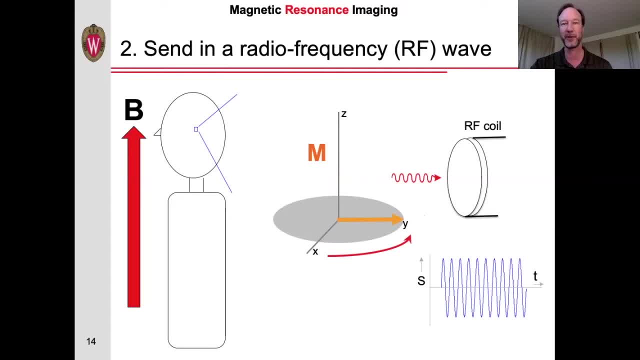 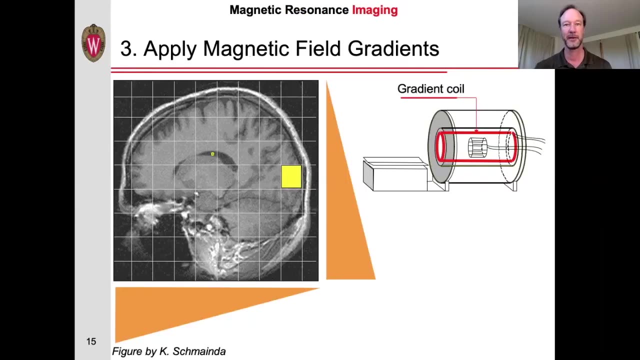 This received coil can either be the same coil as used for sending in the wave or a different one. The amplitude of this radio wave tells us about the amount of magnetization and thus the amount of hydrogen protons or water in the body part we are imaging. 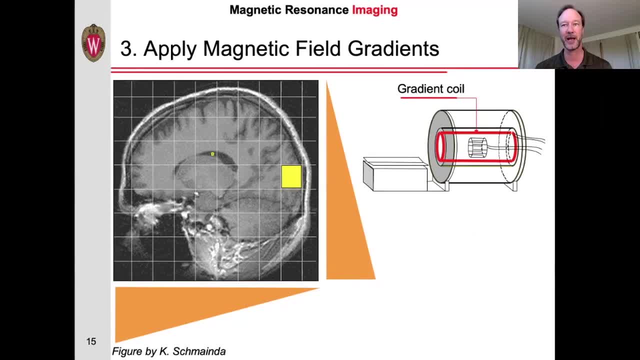 The third step in MRI, the imaging is the magnetization. The imaging is to determine how much magnetization, that is, how much water, there is in different areas of the body part. we are imaging, In other words, we want to create an image of this magnetization. 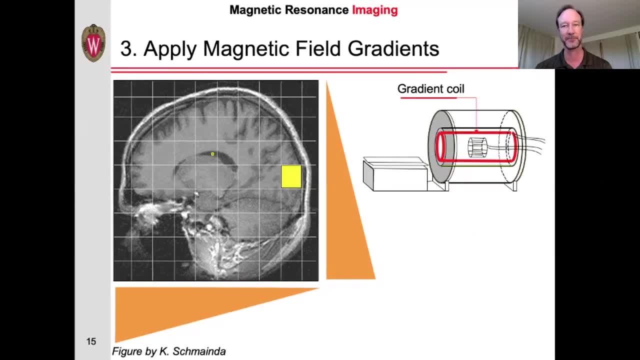 The trick to doing this is to apply magnetic field gradients. As you recall, the spins precess and thus create a radio frequency wave with a frequency that is directly proportional to the strength of the magnetic field experienced by the spins. By making the field a bit stronger on one side of the image, the magnetic field can. 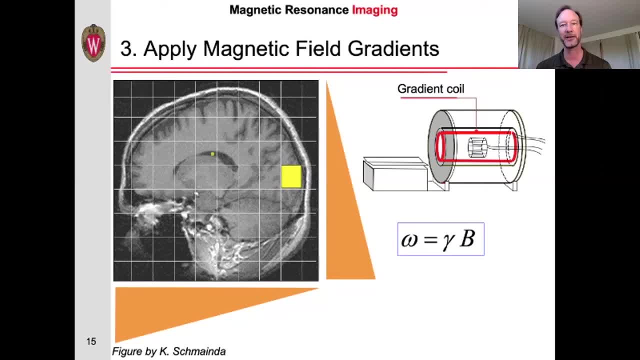 be a bit weaker on the other side. then, by looking at the frequency of this radio wave, we can find out where the signal is coming from. The acquisition is then repeated with different gradients in different directions to build the full 2D or 3D image. 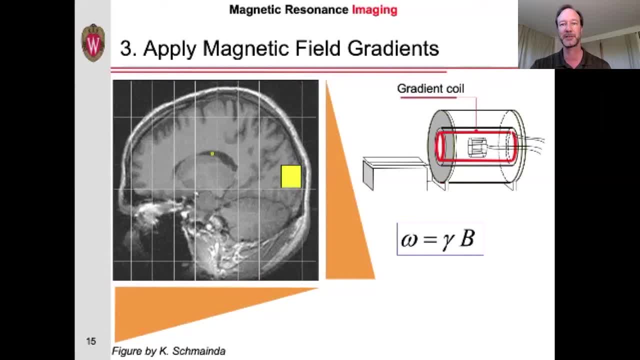 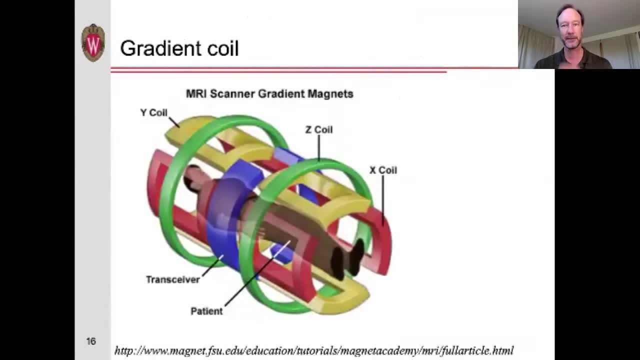 It is largely this trick of using magnetic field gradients to create an image that got Paul Lauterbur and Peter Mansfield the Nobel Prize. Let's take a closer look at how the whole 3D image is formed. The MRI scanner contains 3D images. 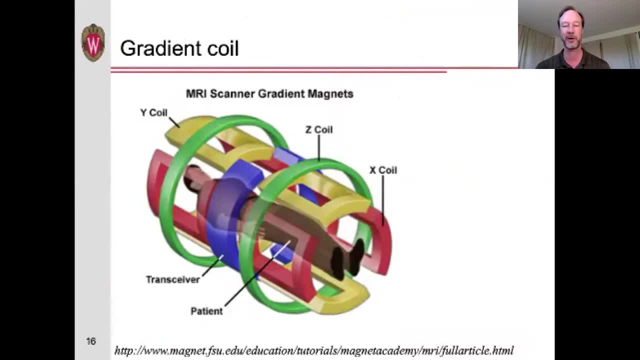 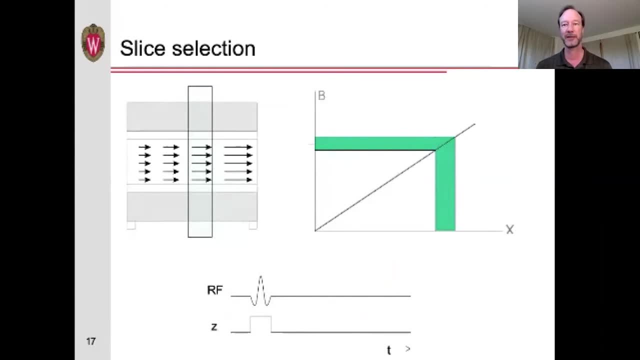 There are 3 sets of coils that can produce magnetic field gradients in 3 orthogonal directions. One way to get a 3D image is to acquire a set of two-dimensional slices. We can obtain data from just one slice by applying a magnetic field gradient in that. 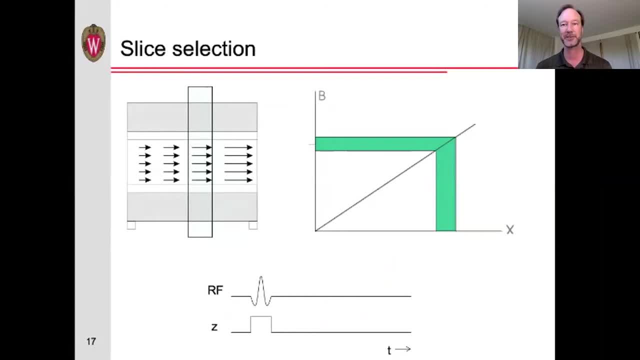 direction while we send in the RF pulse. As I mentioned earlier, the RF pulse will excite the spins if the frequency of the radio wave matches the precession frequency of the spins, The idea of resonance. So if we apply a magnetic field gradient during this RF pulse, only those spins whose 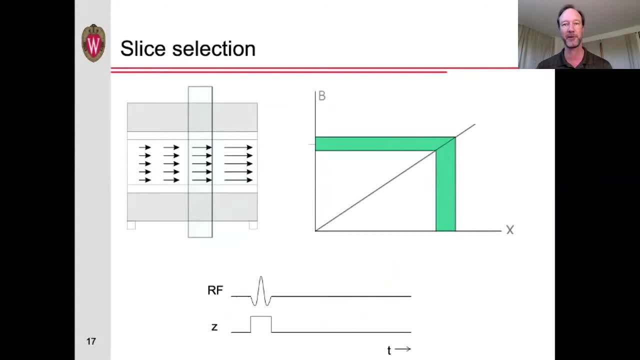 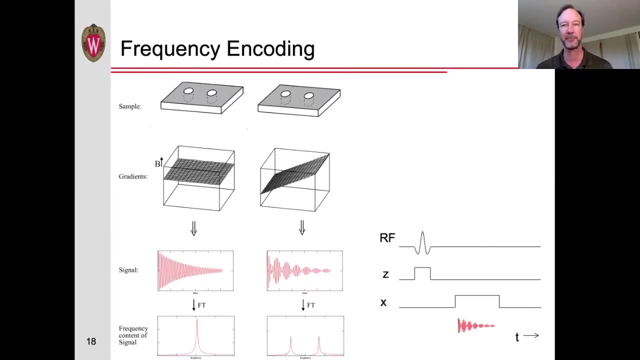 precession frequency matches. the band of frequencies in the RF pulse will be excited. that is tipped into the transverse plane. We can control the thickness of the slice by either varying the gradient or the bandwidth of the RF pulse. Once we've excited that slice, we can encode a second direction by applying a magnetic 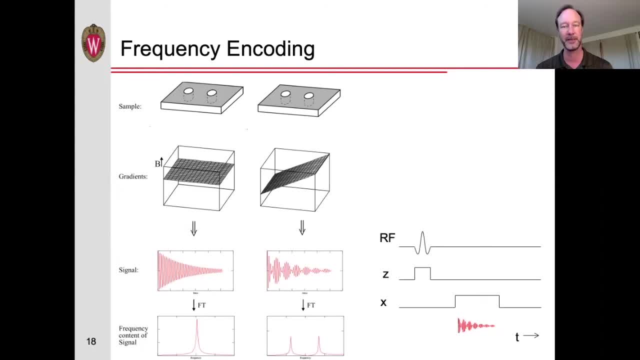 field gradient in that direction while we acquire the data. Imagine we have an object that consists of two tubes of oil. We can then apply a magnetic field gradient in that direction while we acquire the data. Imagine we have an object that consists of two tubes of oil. 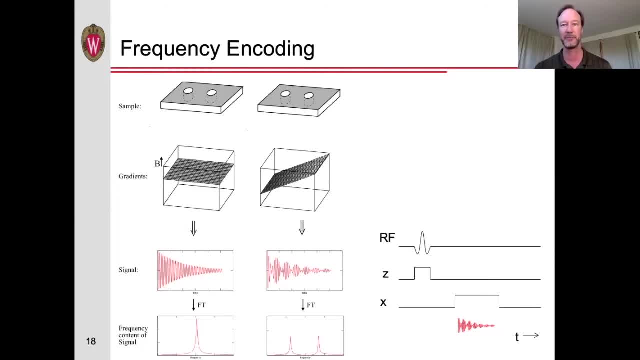 Here I have two tubes of water. If these are in a constant magnetic field, both experience the same field and thus have the same frequency of precession. However, if we apply a magnetic field gradient, the two tubes of water will experience different magnetic fields and thus our spins will be precessing at different frequencies. 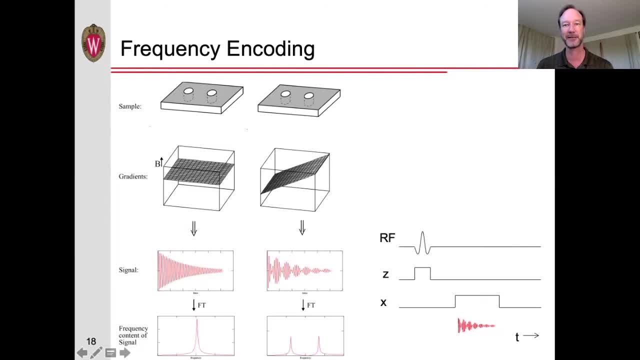 If we look at the frequencies within this combined signal, we can tell where the signals are coming from. And the way we look at what frequencies are in the signal is by applying a Fourier transform. Therefore, if we apply a Fourier transform, these two ambassadors at the degrees limit. 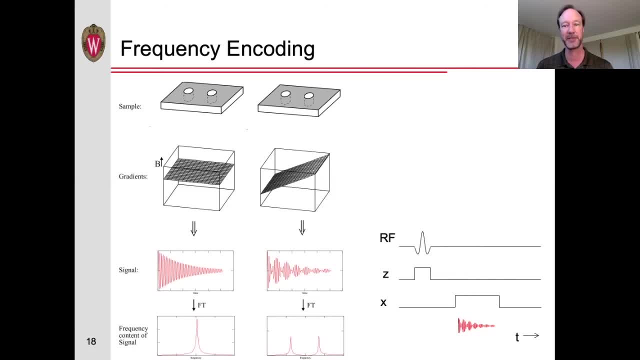 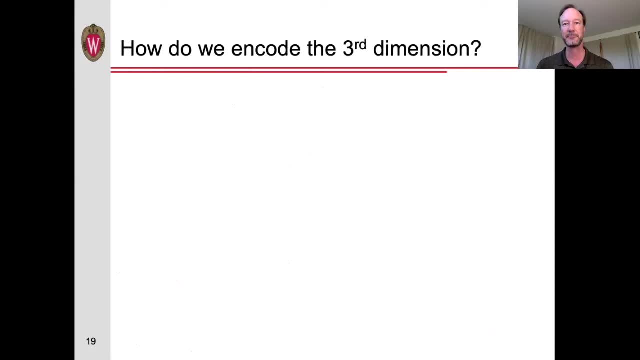 of the magnetic field and thus a specific frequency of precession. If we apply more regular magnetic field, we see that the two tubes of water in a constant Fourier transform to our measured signal. we get an image in that direction. So how do we encode the third dimension? 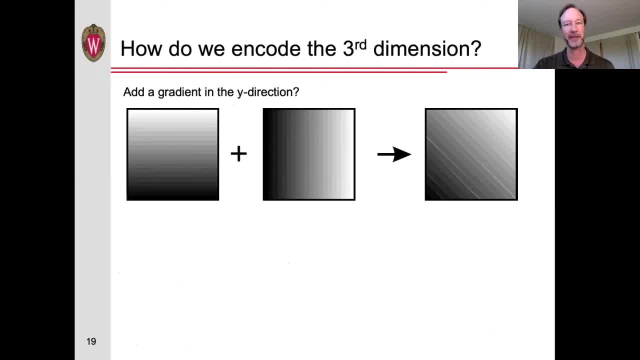 If we apply two gradients at the same time, one in the x-direction and one in the y-direction, it just results in a new gradient in the xy-direction. So that just allows us to see where the signal is coming from along that axis. 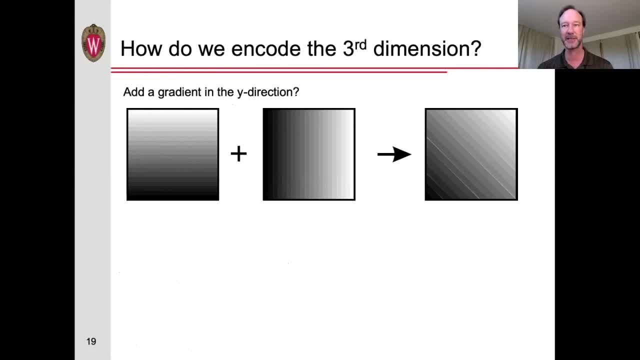 However, if we repeat this process multiple times, and each time varying the x and y gradients, we can use these set of signals, each of which is essentially a projection of the image perpendicular to that axis, to reconstruct the image, a technique that's called projection. 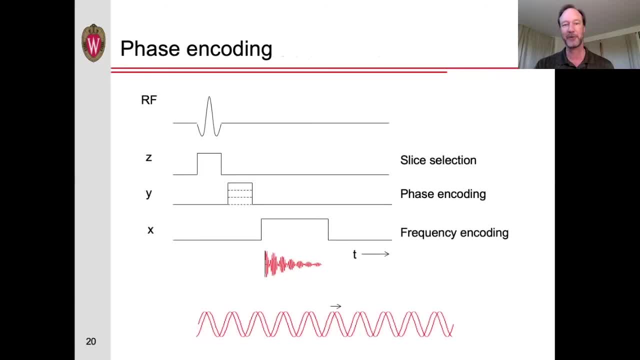 reconstruction. However, a more commonly used way is what is called phase encoding. Instead of applying a gradient during the excitation or during the acquisition, we can apply a gradient for a short time in between the two. This additional gradient shifts the phase of the signal being measured. 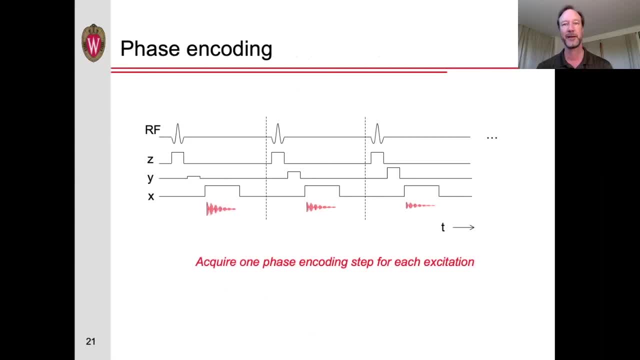 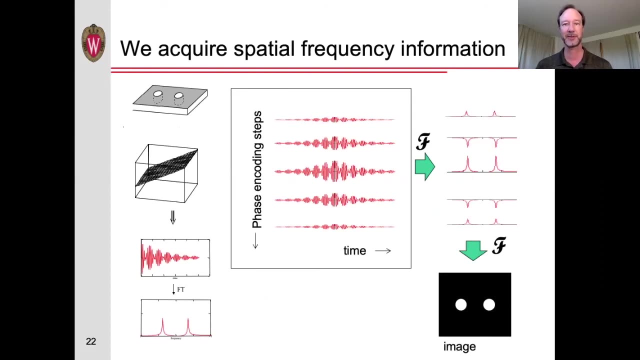 We then have to repeat this procedure multiple times, each with a slightly different amplitude of the phase encoding gradient, and use a set of these signals to form a 2-D image If we stack the set of these acquired signals each at a different phase encoding gradient. 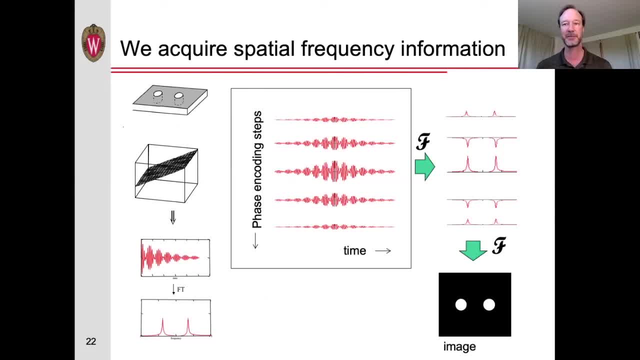 amplitude. then if we look at the frequencies in each of those signals in the x-direction, we can get an image in the x-direction. And similarly, if we look at the frequencies in the y-direction across different phase encoding steps, we can get our image in the y-direction. Now this concept is: 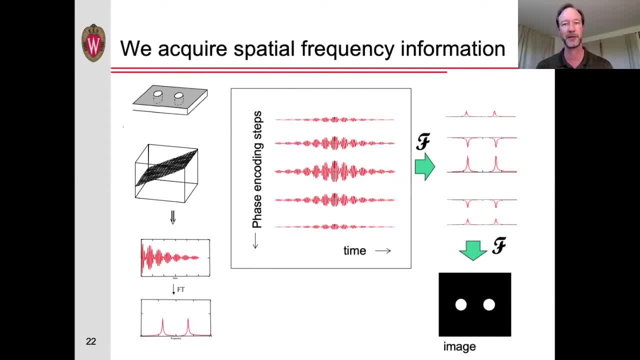 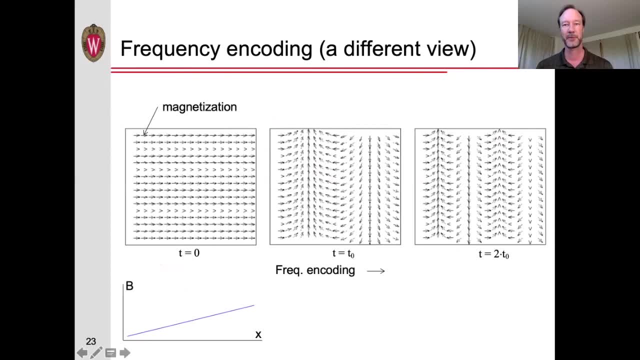 often difficult to understand- at least it was for me when I was first learning about MRI. so let me break this down in a slightly different way. With frequency encoding, we apply a magnetic field gradient while we acquire the signal. If we look at the magnetization in different parts of the image as 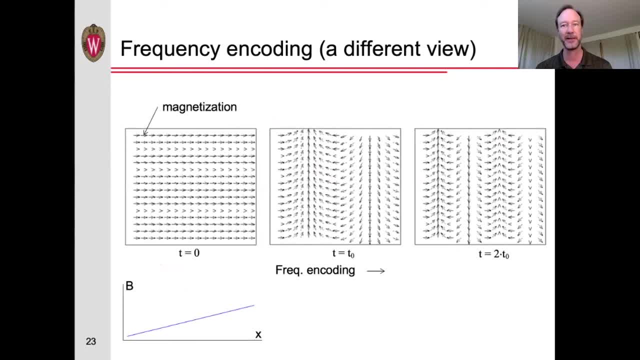 represented here with these set of arrows. then initially, after excitation, all of the spins are pointing in the same direction. But a short time later the spins farther along in the x-direction will be processing a bit faster and will have gotten ahead, while those in the 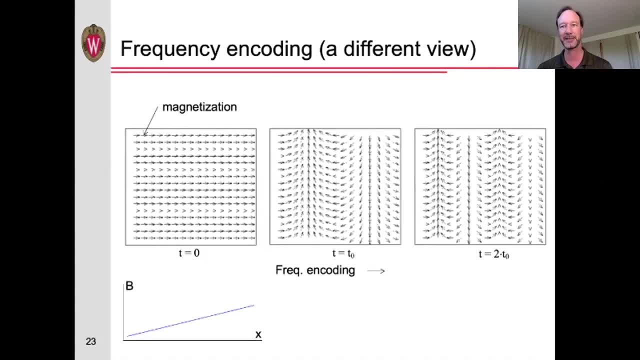 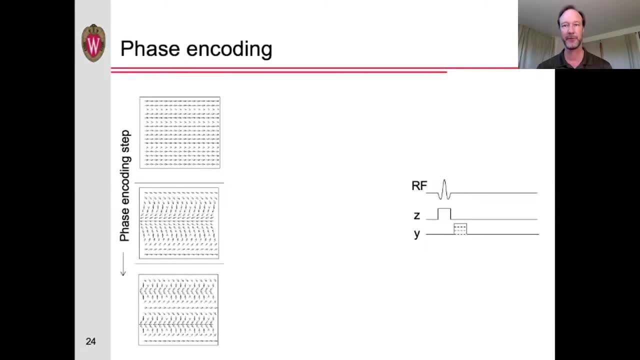 opposite direction will have gone more slowly. So over time the magnetization vectors are getting twisted up in the x-direction. Now let's look at phase encoding. If we don't apply any phase encoding, then when we acquire the data, all the magnetization vectors are still pointing in the same direction. If we 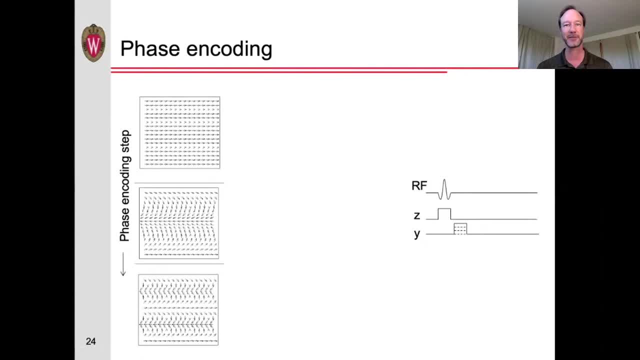 apply a phase encoding, all the magnetization vectors are still pointing in the same direction. If we apply small phase encoding gradient, then the magnetization vectors are twisted up along the y-axis. If we apply an even stronger phase encoding gradient, the magnetization vectors are even more twisted up. 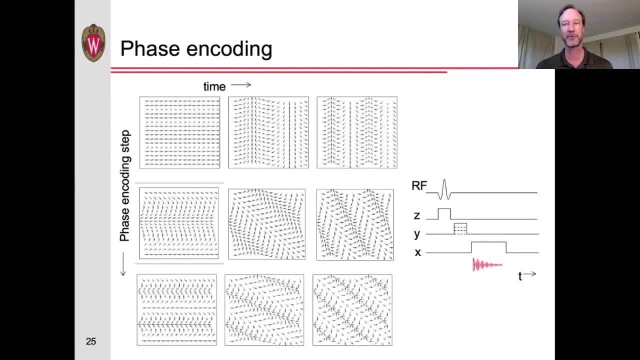 When we then acquire the data. the top row shows what happens without any phase encoding. the second row shows the data when we acquire with a small amount of phase encoding, and so on. Note that how the magnetization vectors are twisted up in the first column is very similar to what is going on in the first row, except. 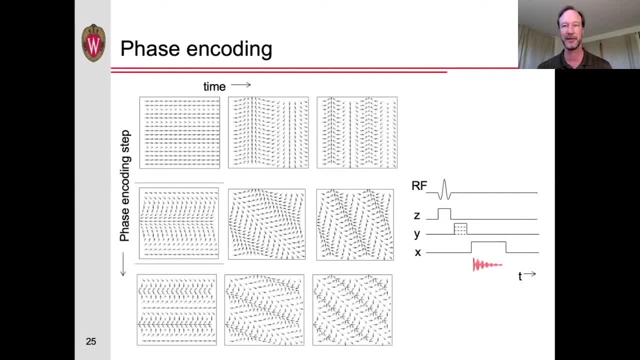 that the twisting is in the y instead of the x-direction. In this way, just as we can find out where the signal is coming from in the x-direction, by looking at the frequencies present in the signal acquired in these rows we could find out.